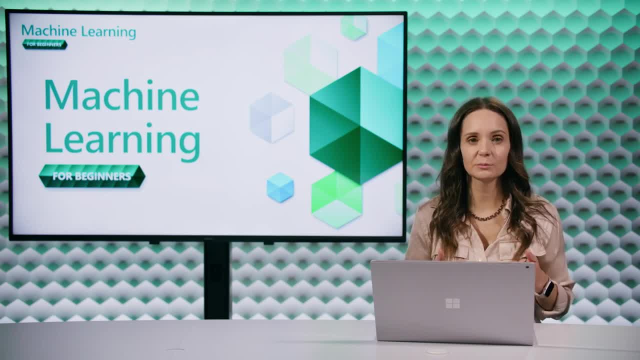 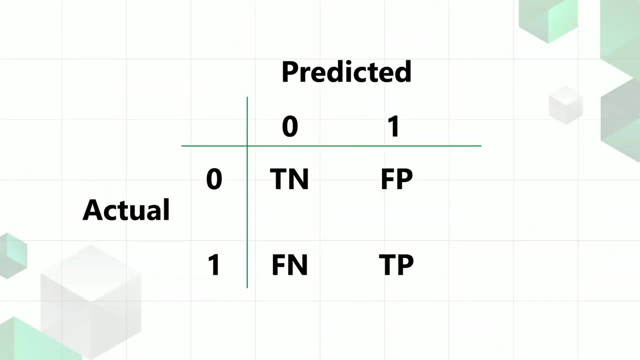 In our scenario, this means that output values smaller than 0.5 that get classified as orange, otherwise they get classified as white. But we can choose a different threshold and if we do, that will impact the results of the confusion matrix. Remember the confusion matrix? We learned about it. 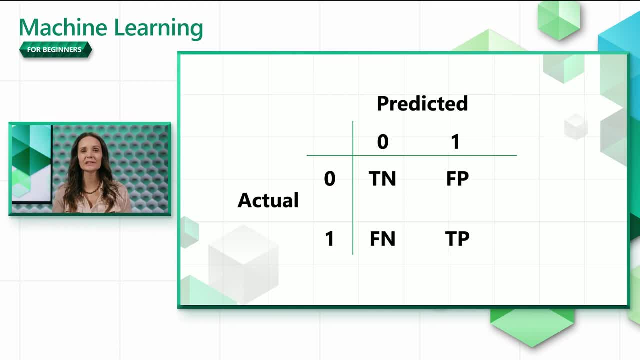 in our last video, but let's look at it again. We'll learn how to calculate many different metrics using the confusion matrix For the ROC curve. we'll need to consider the true and false matrix. We'll need to consider the true and false matrix For the ROC curve. we'll need to. 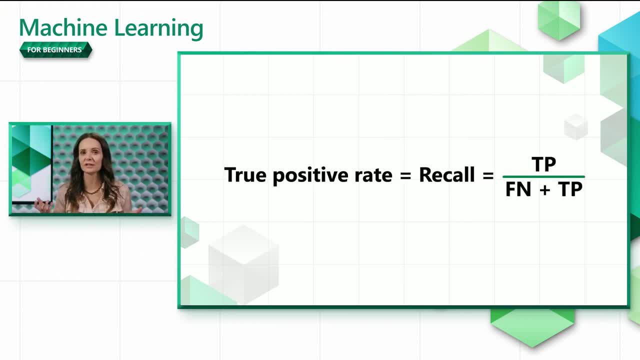 consider the true and false matrix. We'll need to consider the true and false matrix. We'll need to consider the true and false matrix. We'll need to consider the true and false Şimdi Jewel and the true positive ratees. The true positive rate is just another name for recall. 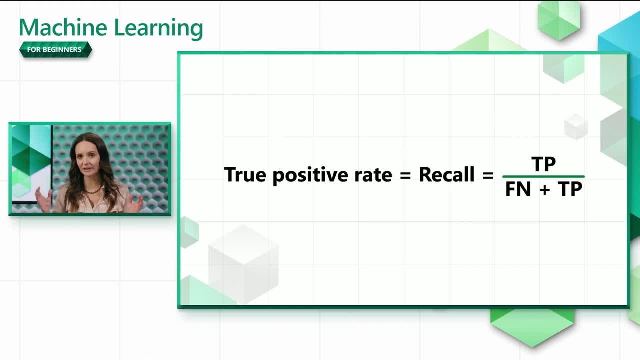 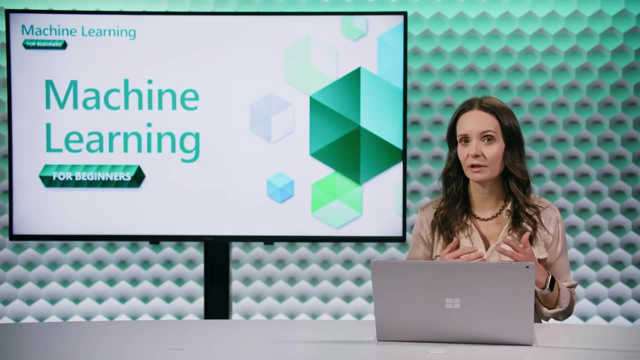 which is the fraction of packages we correctly predicted, as white out of all packages are actually white. The false positive rate is the fraction of orange packages were incorrectly predicted, as white out of all packages are actually orange. To draw an ROC plot, we consider a classification. 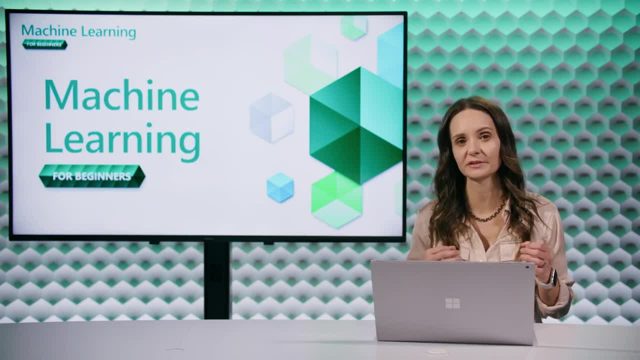 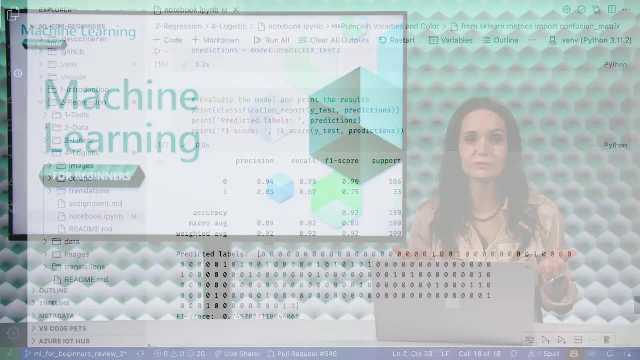 threshold value, We calculate the corresponding true and false positive and we add a new point to the plot, using the true positive rate as the y value and the false positive rate as the x value. Then we repeat for several different classification thresholds, eventually ending up with a curve. Doing this in code is a bit simpler: we just need to call the: 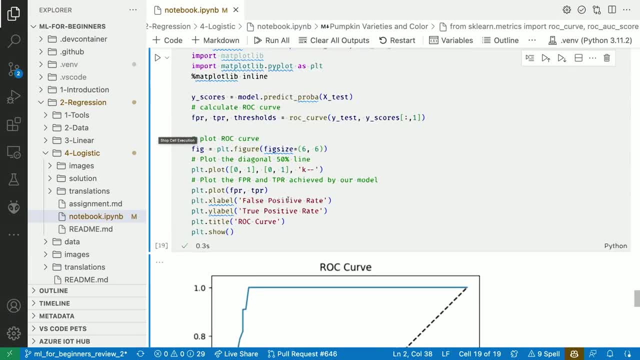 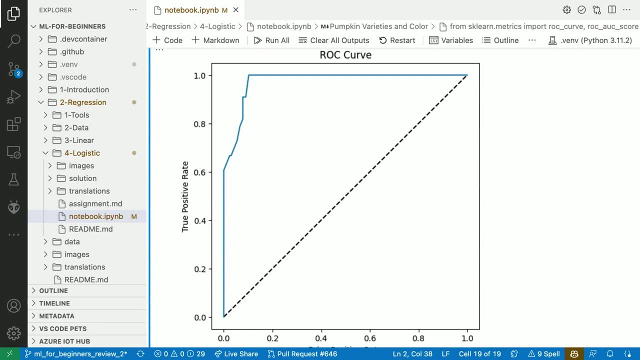 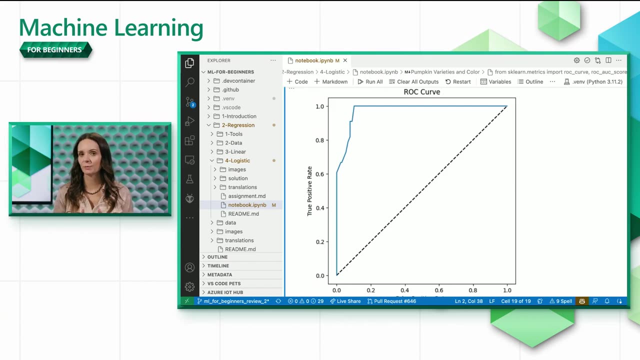 roc curve function and give it our actual and predicted labels. We get back lists containing the false positive rates, true positive rates and the thresholds, and we use the first two to plot our curve. Let's think about the shape of the roc curve for a moment and see how it relates to the 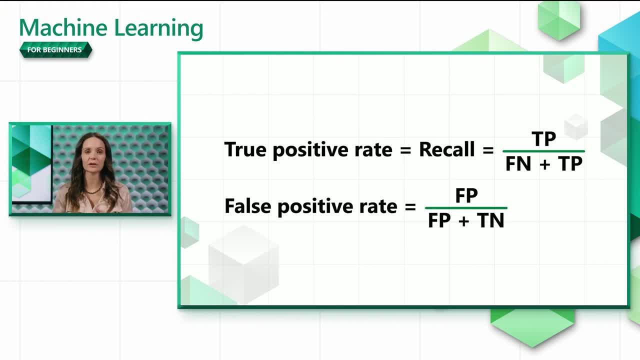 formulas. If our threshold is zero, then we classify all inputs as positive, because we don't have any values classified as negative. our true positive and false positive rates are both one. On the other hand, if our threshold is one, then we classify all inputs as negative. 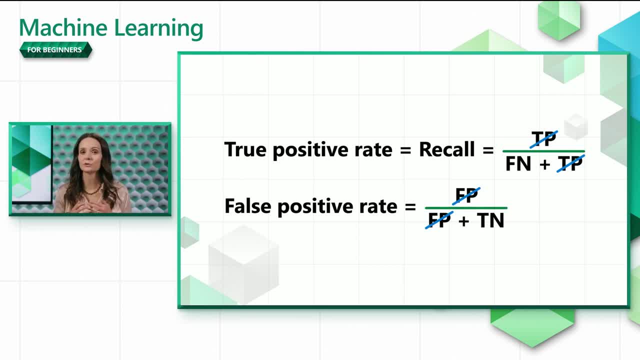 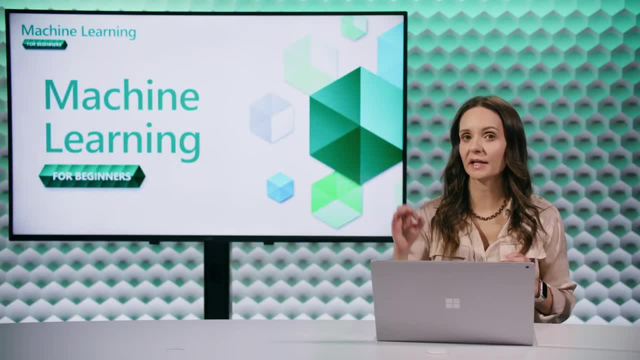 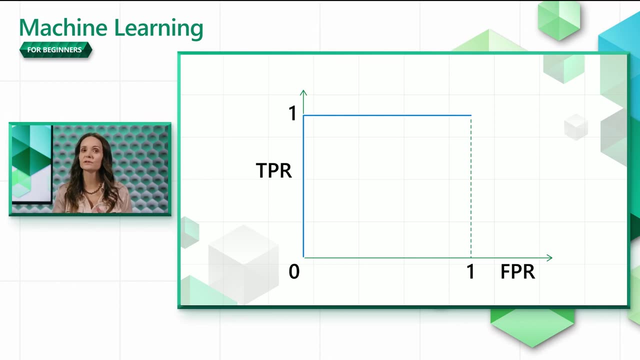 Because we don't have any values classified as positive. our true positive and our false positive rates are both zero, So our roc plot will always contain the points zero, zero and one one. What happens in between depends on how good your predictions are. Ideally, we want the true positive.